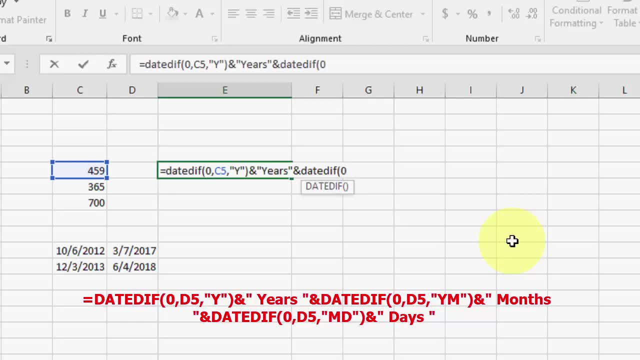 open the bracket zero comma. select the y dates or dates and then comma: open quotation y, m. close quotation bracket and type and open quotation months. close the quotation and type and symbol again type date. if open bracket zero comma, select your cell like this: Comma md, sorry. open the quotation type md. close the quotation. close the bracket and type and symbol. open the quotation type days. close the quotation and hit data. boom, that's it. 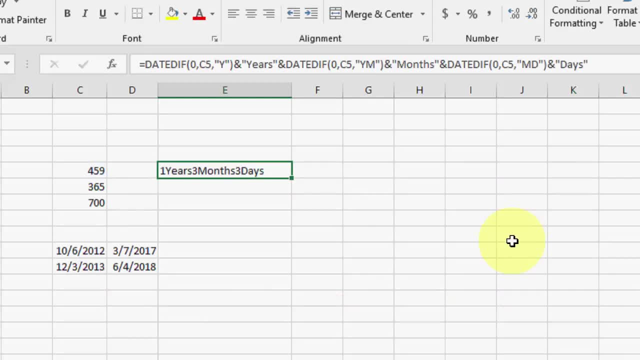 So we got the total years, month and date. It's looking a little disturbing So you can take the space. So, for the time space just here, your life is before, In eight, after the ears like these, months like this and dates like days. Okay, So here. 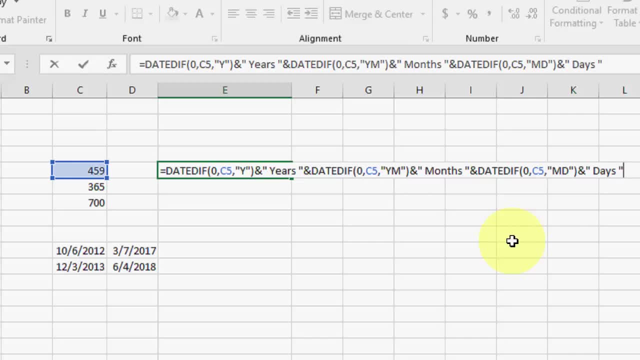 we got the clear, everything Okay. So if you feel any difficulty, right this formula. I have given the formula in my video: 6000. just copy and paste. Yes, you need to change this. you are saying number, so change thiszia Highway Number as per yourself and you'll get this. So this is that convertach. just copy and paste and paste your cell number. That's doubleی. 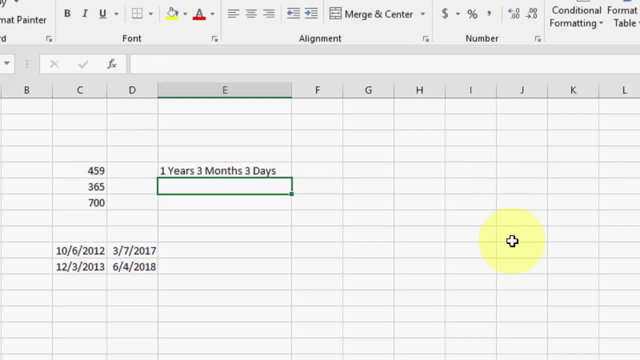 ikes are. check every here And test these numbers when asking the channel most summary. You are right, are meeting these? somebody over pepperpan by see what weight of time And you will get the results. So this is that. convert it. just copy over all multiple people. Quite it well, this sweetly. just call to ask the debtist. You will receive your key to unless. choose this this themselves. if you want to enter, STOP taking this. 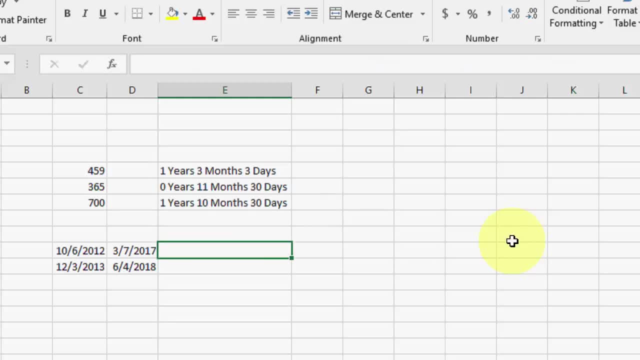 paste for other thing like this. okay, now how to convert date in between. so, for example, i have this: a date from 10, 6, 12, 2, 3, 7, 17.. so for this you need to write the simple formula, not a simple. 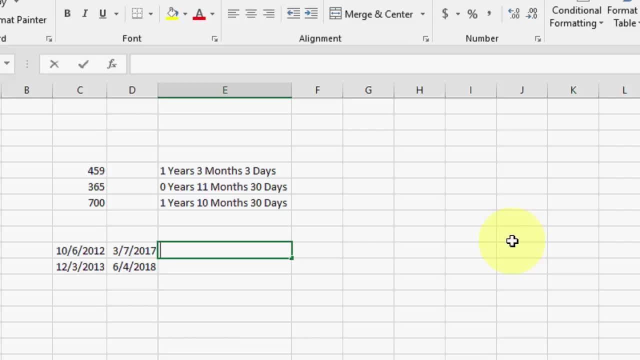 it's a lengthy formula so, as i said, you can copy paste. just type is equal to okay and type dated. if open the bracket and select your cell like this, this cell is returned to return like this: select this and comma, give the comma okay and type in the red comma y, close the inverted comma. 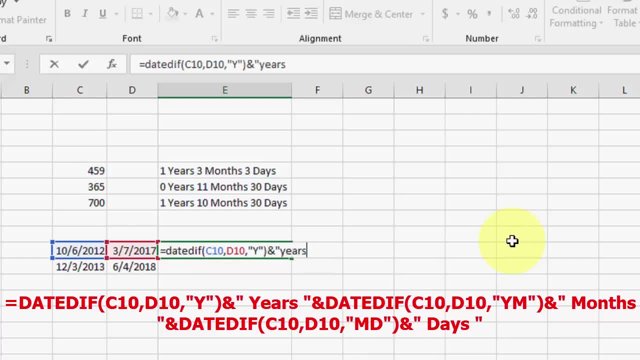 close the bracket. type iron icon and now type ears- okay ears. close the inverted comma and type iron icon. then data. if open the bracket type search, select your data like this: close this in red comma. or you can say quotation: open the quotation and type ym. close the quotation. close the bracket. insert the end icon. 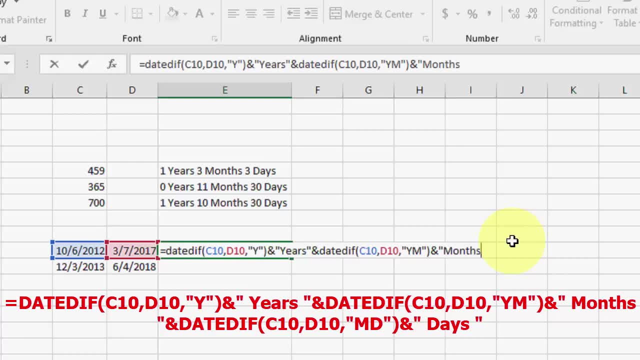 type month. sorry, open the inverted comma. type month. close the inverted comma and here insert the end icon. now type date it. if open the bracket, select your cell like this: okay, now open the quotation type md. close the quotation. close the bracket. insert the icon and icon and open quotation days. close quotation and hit enter. boom, that's it. so we got the result. 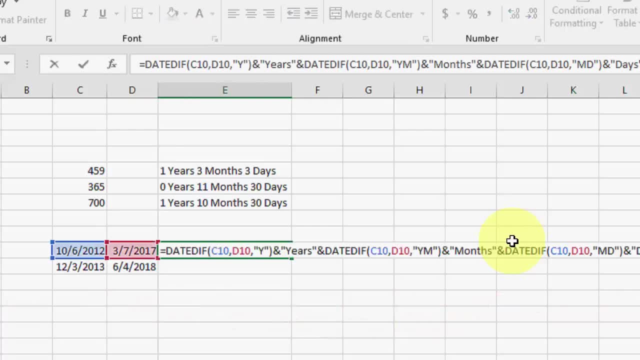 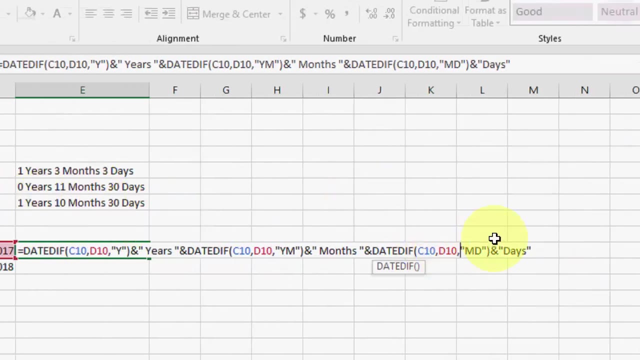 so it's looking little uh confusing. uh, you know this is an example, so, like this, what we prefer is uh confusion. so for this you can give space here in the year section. give before and after my space, like this year, month, okay, and the dates you want, the space before and after. 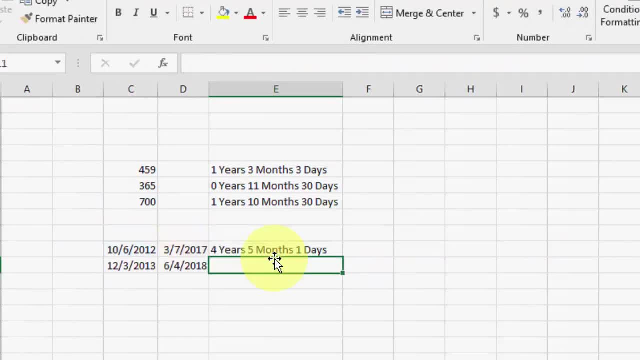 and now i change her and boom, we got the result. so this is the- uh, some confusing formula. so don't worry, i have given this formula in my video. just copy the formula and just you need to change your cell number, this cell number. just just change the cell number and you are. 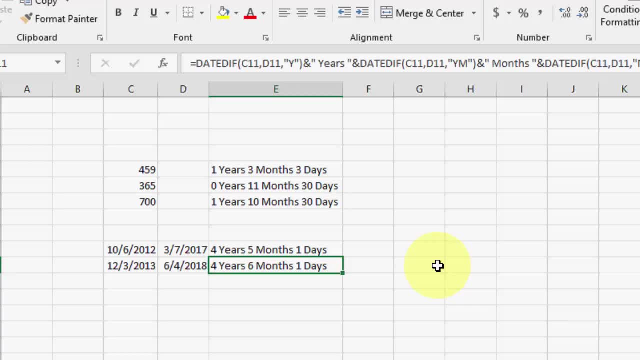 good to go. that's it, man. so just you can apply this to all your other worksheet. so that's it. thanks for watching, guys. if you have any question, you can ask in comments, or if you have any shorter idea or shorter tip to do this, you can share in comments. 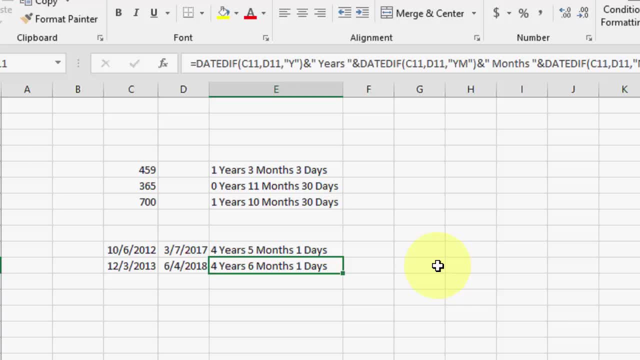 thanks for watching guys. catch the next video. please like share and subscribe. thank you very much.